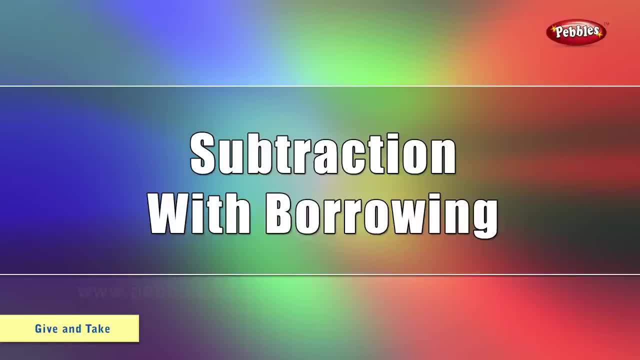 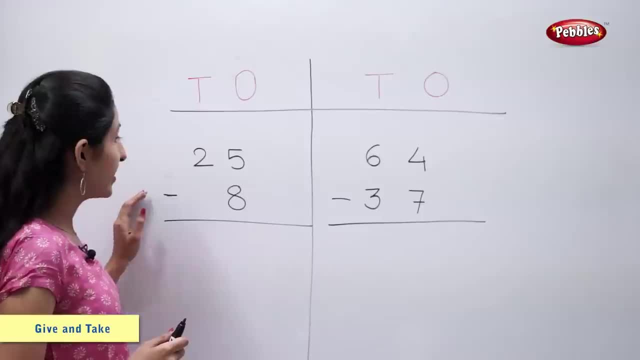 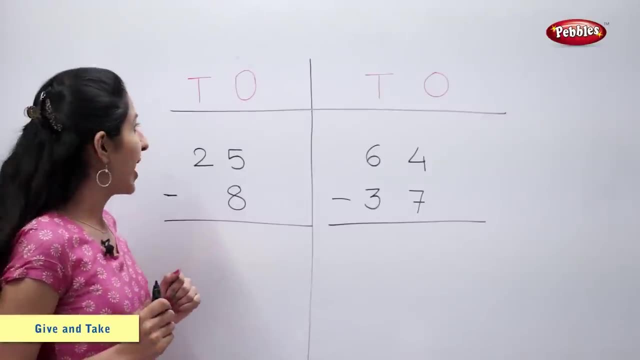 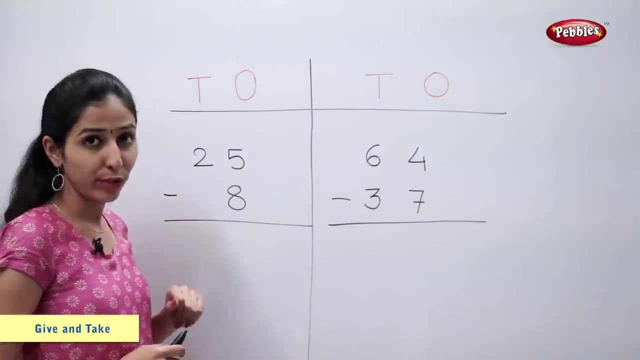 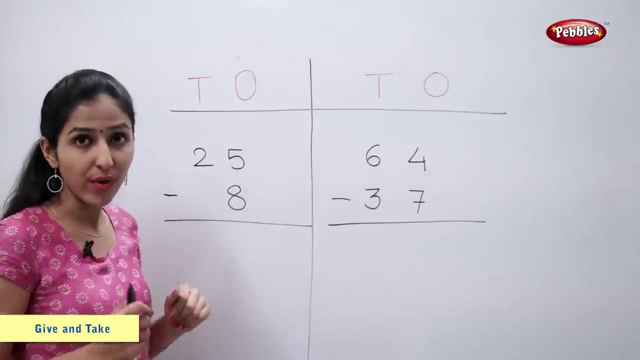 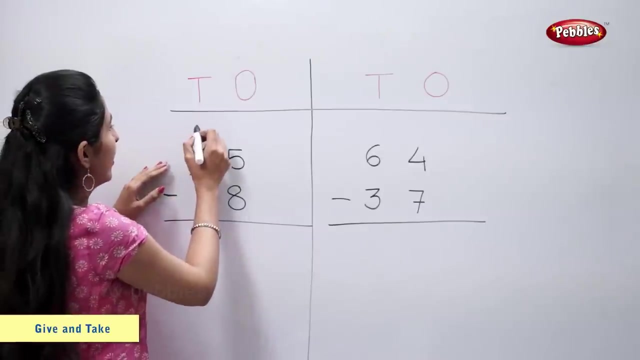 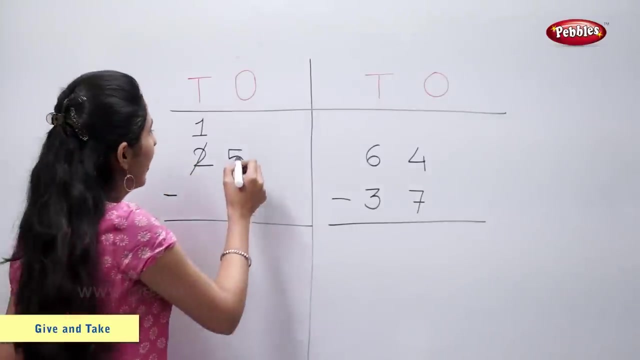 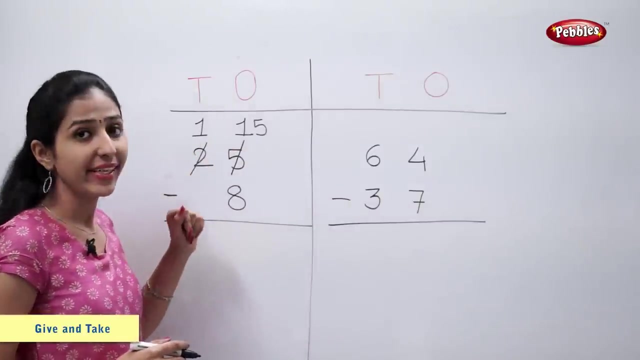 Subtraction with borrowing. Let's look at these examples: 25 minus 8.. Let's find out how much is 25 minus 8.. Let's subtract ones first: 5 minus 8.. Students, we cannot subtract 8 ones from 5 ones, So we will borrow: 1 tenths 2 becomes 1.. 5 becomes 15.. 1 tenths 5 ones. 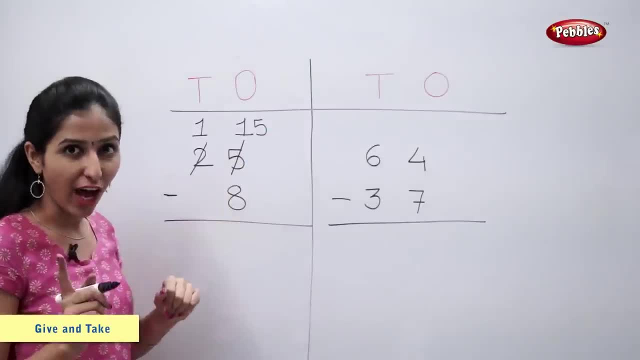 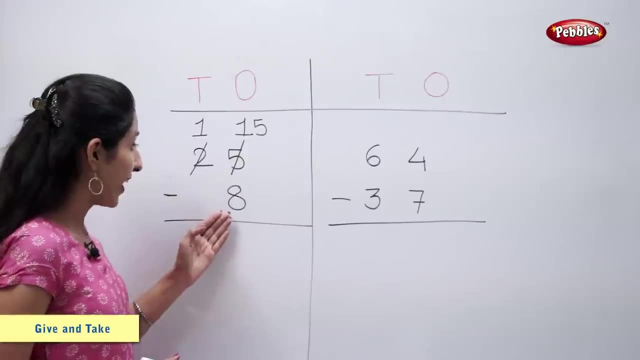 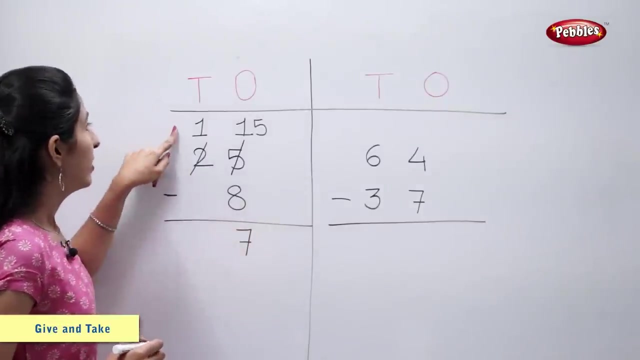 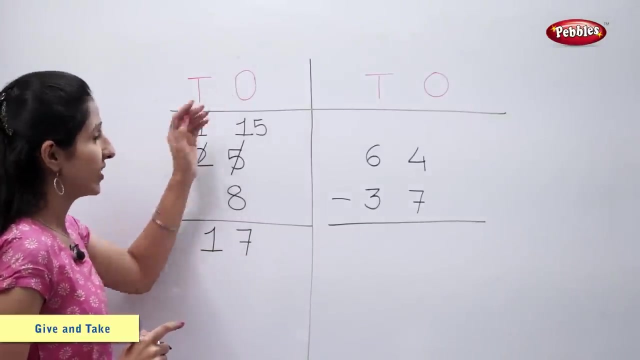 is equal to 5. 15.. Now we can subtract 8 from 15.. 15 minus 8 is equal to 7.. Now this 1 tenths comes down, So we have 1 tenths 7 ones. That means we can subtract 8 from 15.. Now we can subtract. 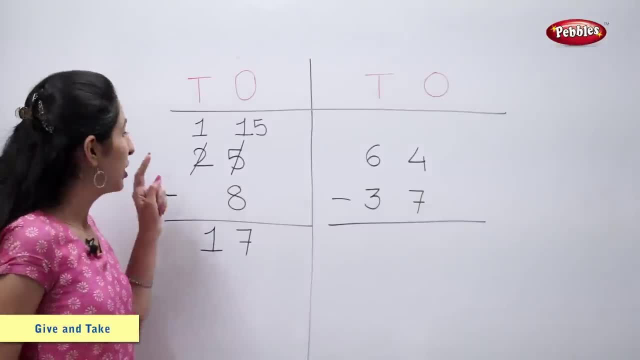 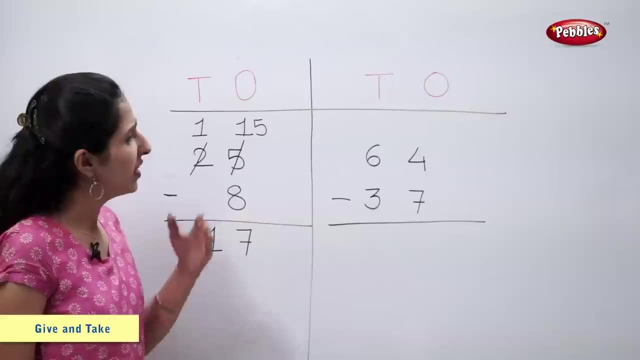 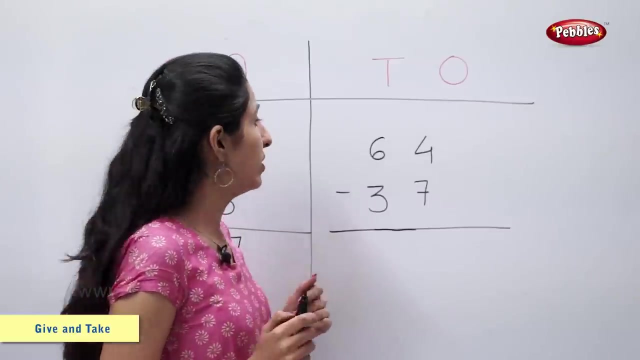 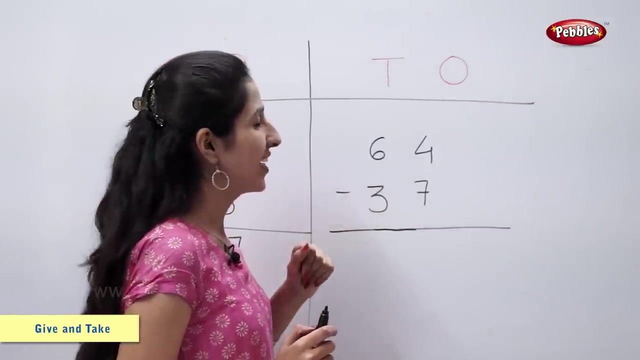 makes number 17.. So 25 minus 8 is equal to 17.. Let's solve this example: 64 minus 37.. Let's find out how much is 64 minus 37. Let's subtract ones first: 4 minus 7.. So 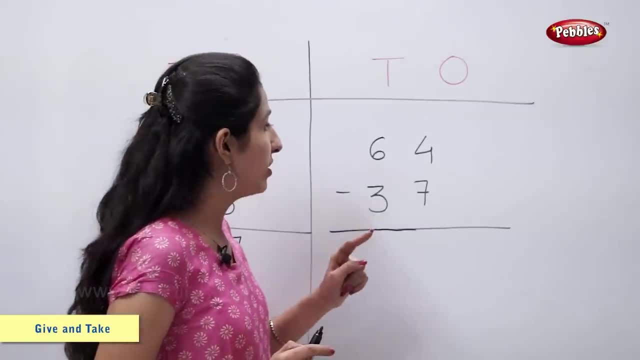 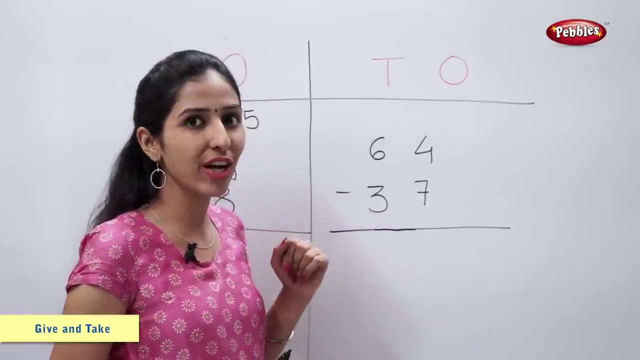 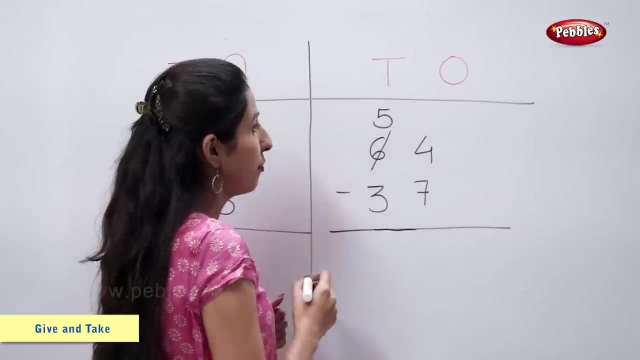 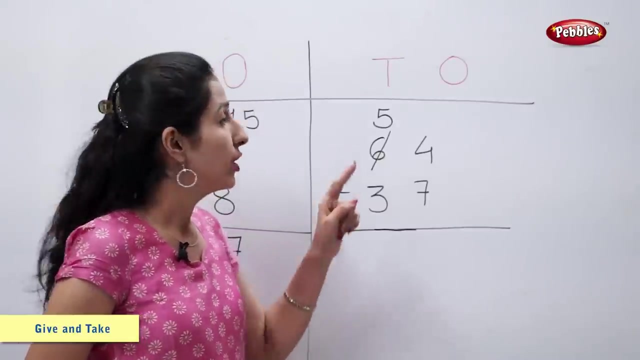 students, we cannot subtract 7 ones from 4 ones, So we will borrow 1 tenths from tenths column. 6 minus 1 is equal to 5.. 4 plus 10 is equal to 14.. So this 4 becomes 14.. Let's. 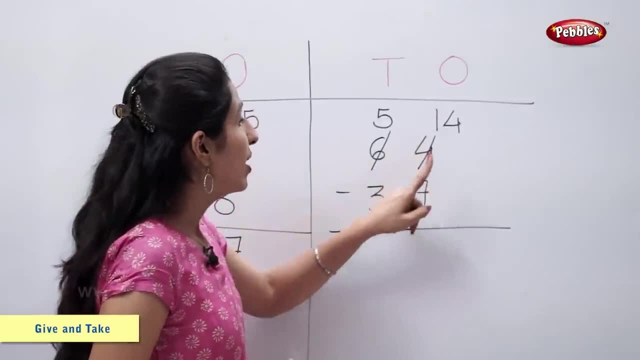 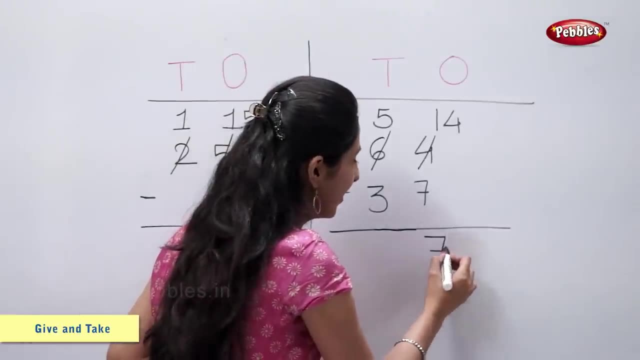 borrow 1 tenths from 5.. 4 1ths from 5.. 4 1 1, 1.. That means that's 5: 1 threes from 5.. Now we have 2 tenths from 10.. So 6 minus 3 is equal toむ. So 1 tenths from 5 is.